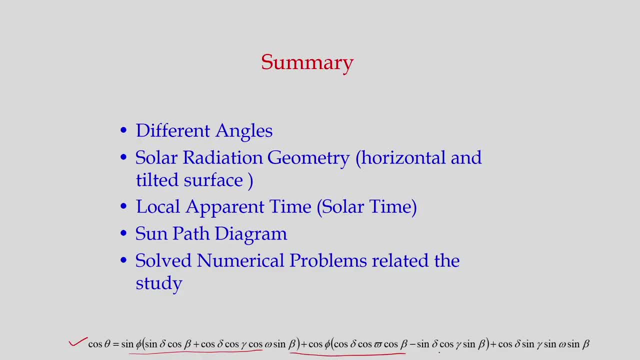 So, as you can see, this theta is a function of difference, And for calculation of omega- that is, hour angle- we have to understand how this local apparent time can be calculated. Once we calculate this local apparent time, then only we can calculate what is omega. 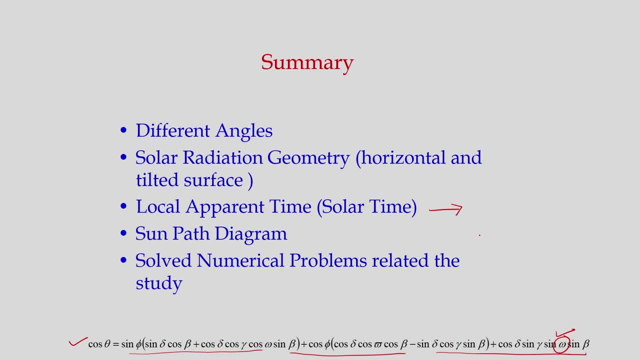 So that also we have discussed And we have discussed sun-part diagram, how sun travels in the sky From the observer and how this variation takes place in case of summer, in case of winter and in case of equinox, And we have studied the solar radiation geometry for horizontal as well as vertical or tilted surfaces. 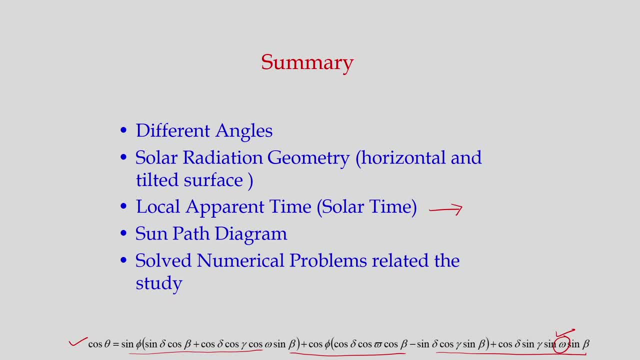 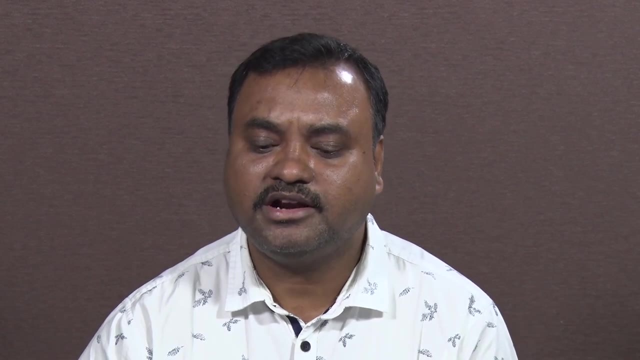 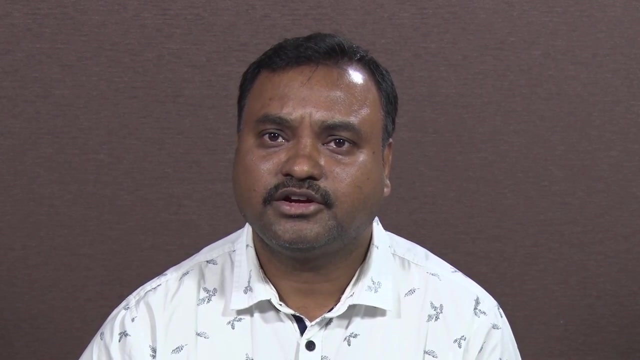 Also, we have estimated the day length by using the calculations And we have solved numerical problems to strengthen our understanding, Thank you. So in today's lecture we will concentrate on estimation of solar radiation under different climatic conditions. Primarily, we will emphasize the monthly average of daily global radiation estimation. 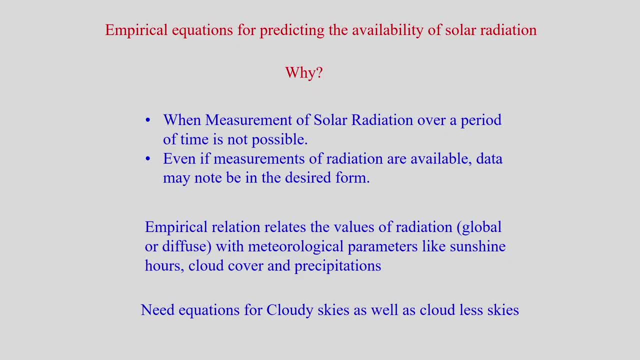 So now, before we start the empirical relationships or correlations, we must know why this kind of correlations are very, very important. The first thing: why we need empirical equations for predicting the availability of solar radiation. So if we have enough solar radiation data by using some kind of devices, then it is well and good. 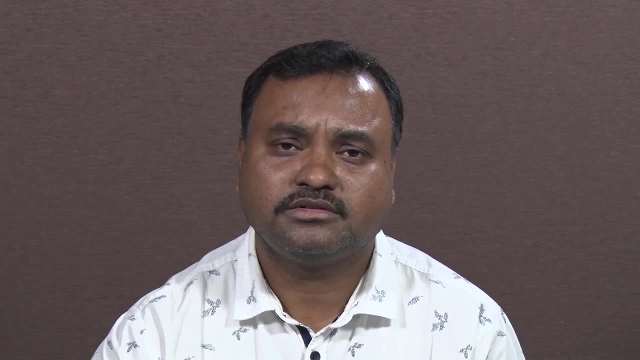 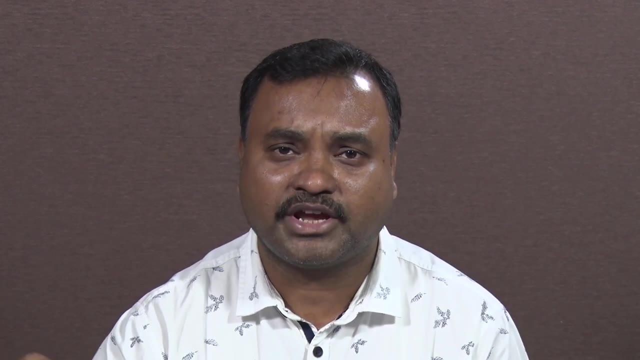 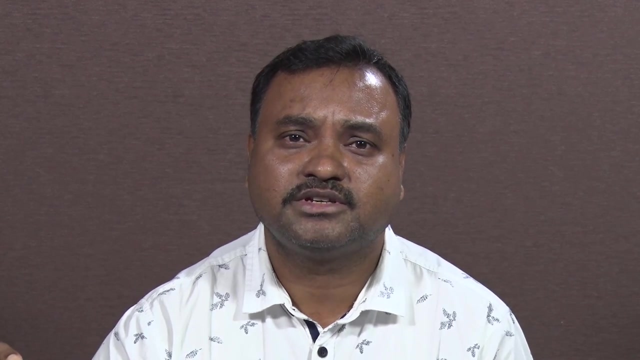 Then we can straightaway use those data for calculations. If this data is not available for a particular location, then we cannot use it for calculations. If this data is not available for a particular location, so where we are targeting to do the calculations, then we will look for some kind of places which is having similar climatic conditions and geographical conditions. 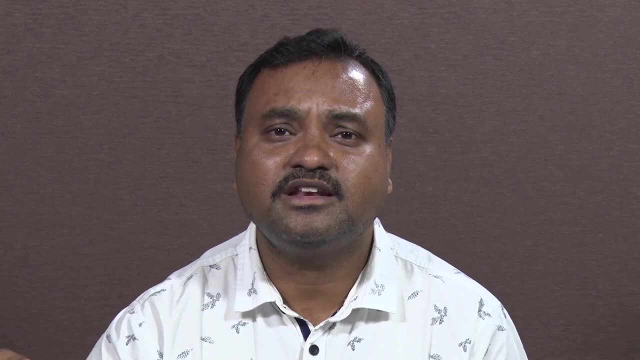 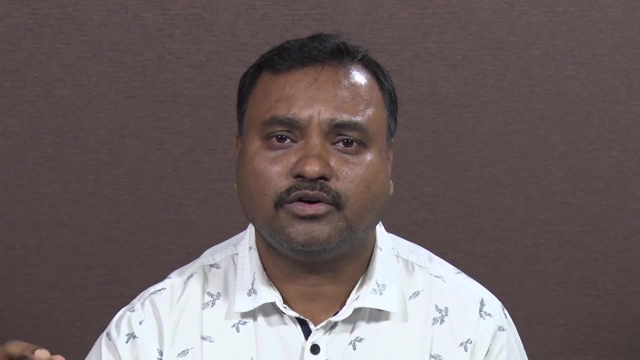 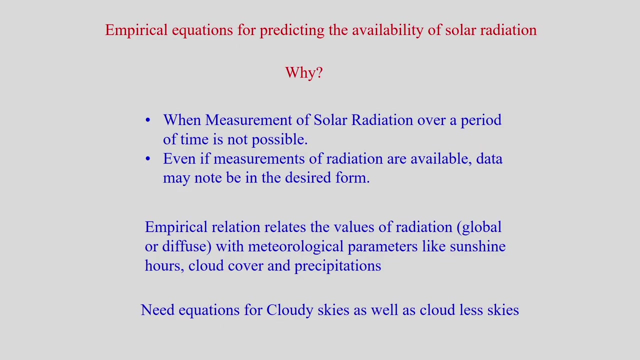 So if this criteria is also not meeting, then we will look for correlations which can give approximate values of the targeted value of the radiation. And sometimes what happens, even though we have solar radiation data we cannot take straightaway because our requirement will be something else. 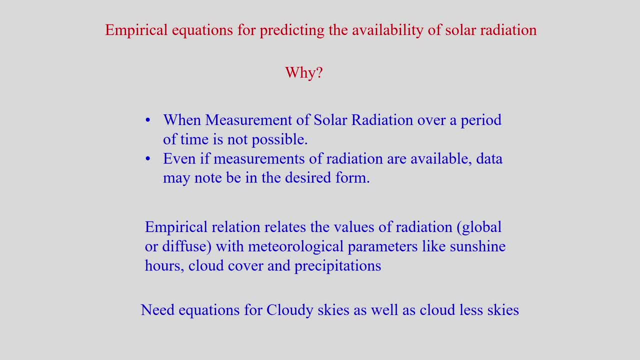 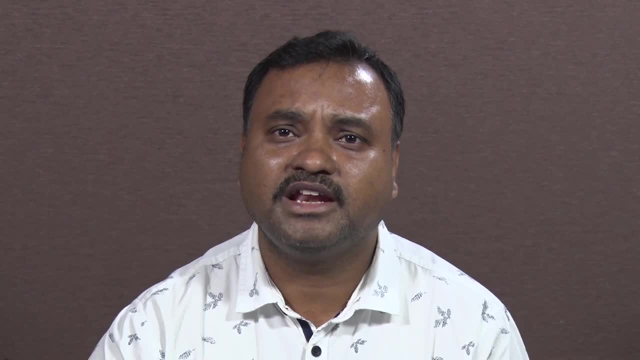 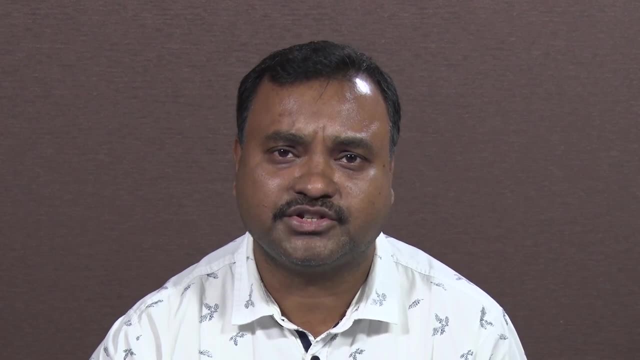 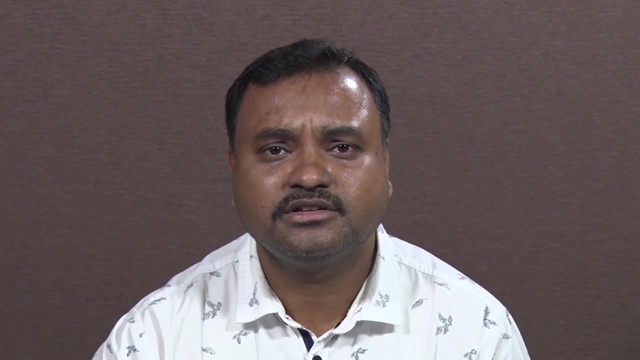 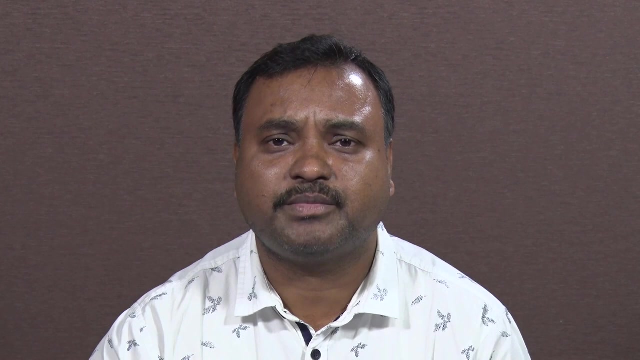 For example, suppose if we get a data from some sources and that is maybe daily variation of global radiations, So it might show even that I need hourly variation of global radiation. So for that we need to do something And sometimes what happens? we have global radiation but we need to know the percentage of diffuse radiation and percentage of normal radiation in the global radiation. 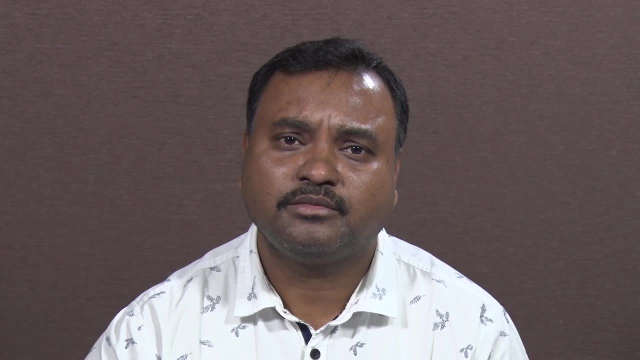 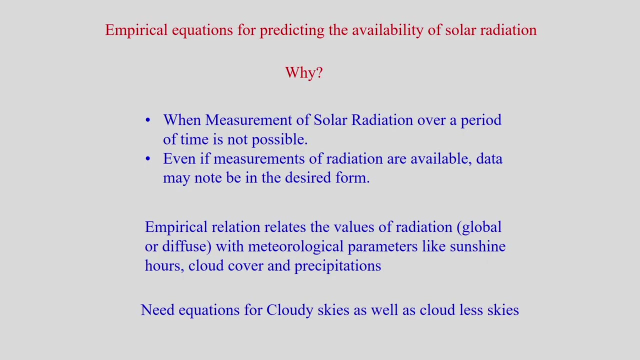 So in order to calculate those parameters, we need to depend on some kind of correlations which relates the radiation data and other meteorological data, something like sunshine hours, cloud cover and precipitations, So that way we can develop some kind of correlations to estimate. 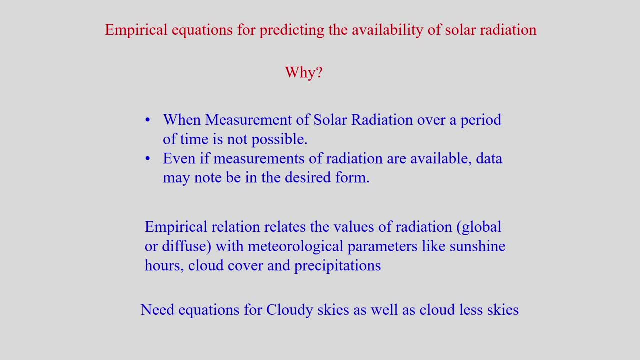 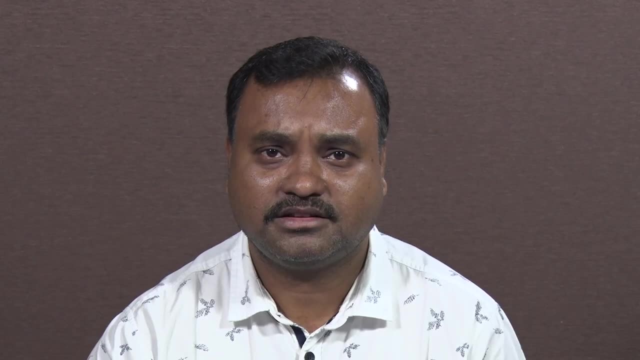 solar radiation data for a particular location. And these correlations what is developed so far by the researchers? these are not the unique correlations. We cannot use a single correlation for all the cases or all the places, So there is a need of development of correlation. 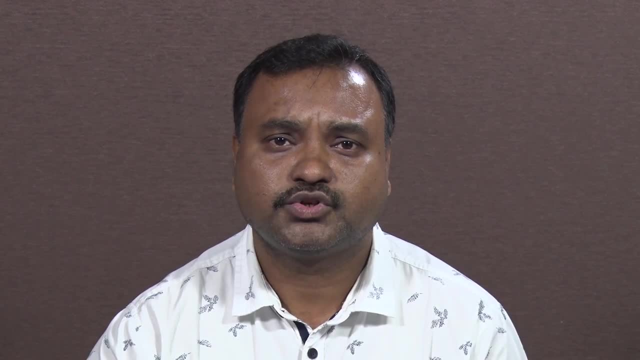 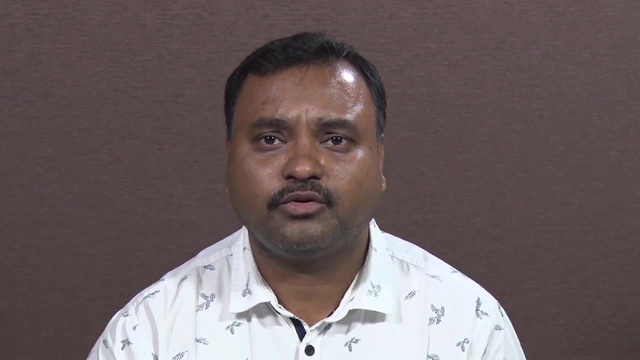 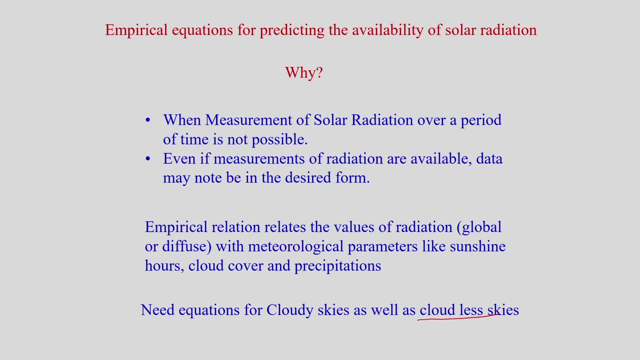 for a specific locations so that accurate estimation of radiation can be done. So we need to have different correlations for different climatic conditions and that way: again cloudless sky, that is clear sky, and again cloudy skies. So there are many correlations for estimating the radiation under these different climatic conditions. 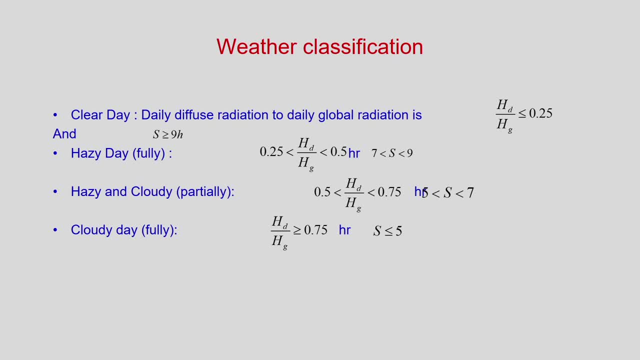 Also, some of the researchers claim that we can classify the weather in different classes, like clear day, hazy day that may be fully hazy. hazy and cloudy that is partially, or that may be cloudy days that is fully cloudy. So that defines. 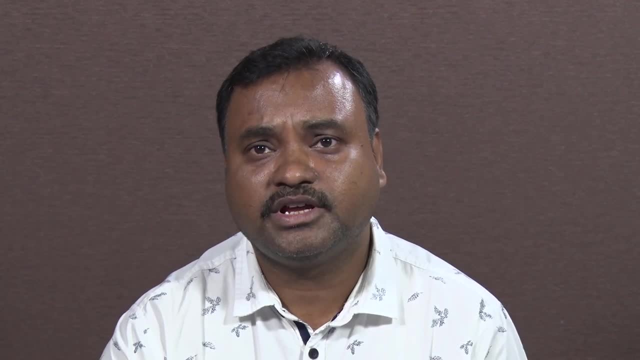 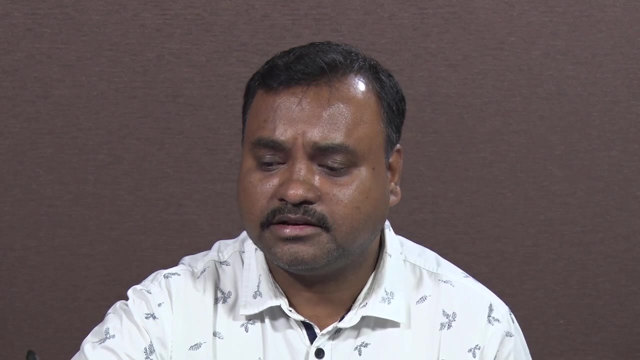 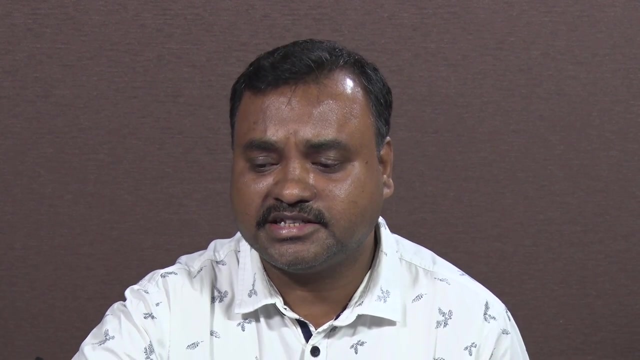 this weather can be classified based on the percentage of diffuse radiation in global radiation. So if we represent the diffuse radiation is hd in a day and global radiation is hg in a day. if it is less than this ratio- is less than 0.25, then we can say it is a clear day. 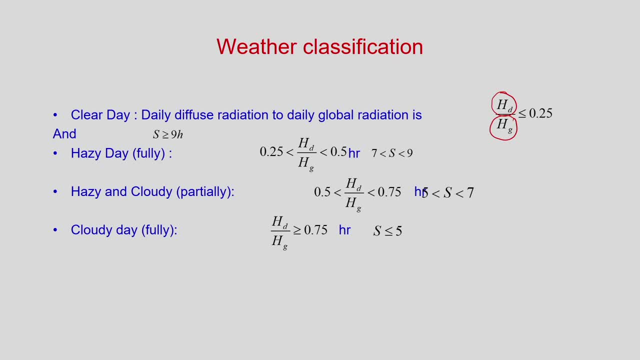 or clear sky. no cloud is there. At the same time, we need to concentrate about the timing, and timing has to be greater than 9 hours. that is sunshine hour. sunshine hour has to be more than 9 hours, So under that condition, we can consider that day is clear day or cloudless sky. 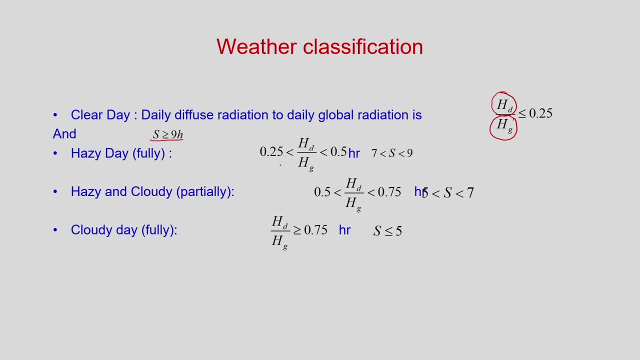 And for hazy day. this ratio is in between 0.25 and 0.5, and sorry this hour should be here. So this timing, or say sunshine hour, should be in between 0.25 and 0.5.. So this timing, or say sunshine hour, should be in between 0.25 and 0.5.. So this 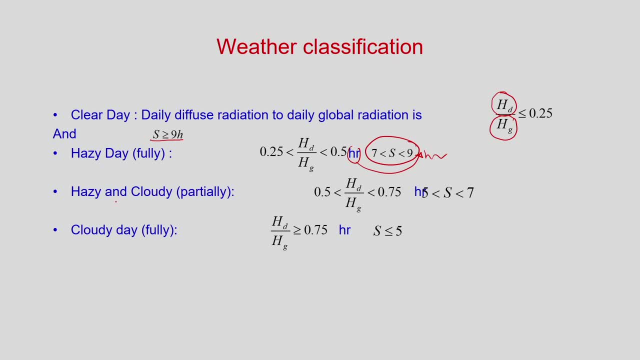 timing, or say sunshine hour, should be in between 0.25 and 0.7, and 9 hours Accordingly. for hazy and cloudy day, this ratio is in between 0.5 to 0.75, and this day length or sunshine hour is in between. 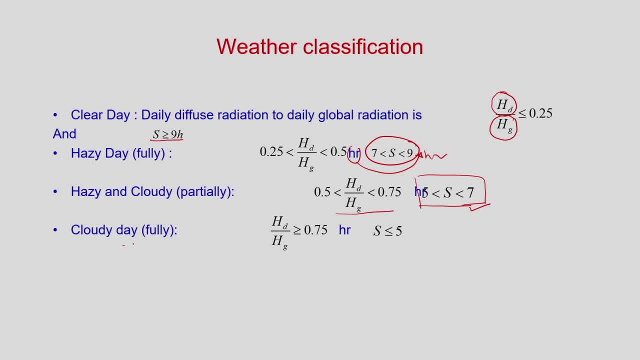 5 to 7 hours And for cloudy day, which is fully cloudy. so this ratio has to be greater than or equal to 0.75, and this timing sunshine hour is less than 5 hours. So under that condition, 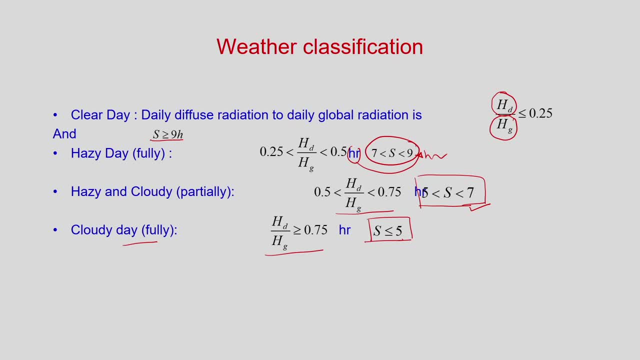 we can have different correlations. So for the time being, what we say? we will classify this as a cloudy day. cloudy day and this we can say clear sky or clear day. no cloud is there. First let us study the correlations developed. 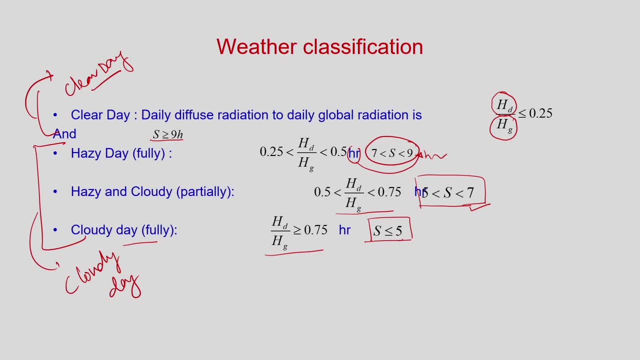 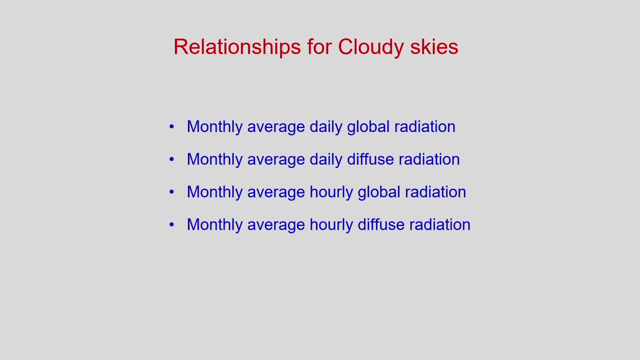 for estimation of monthly average of global radiation for cloudy days. So there are different correlations, as I have discussed, like monthly average daily global radiation. sometimes researchers are required to know for calculation of solar estimations or say solar device installation, that what is the monthly average of daily global? 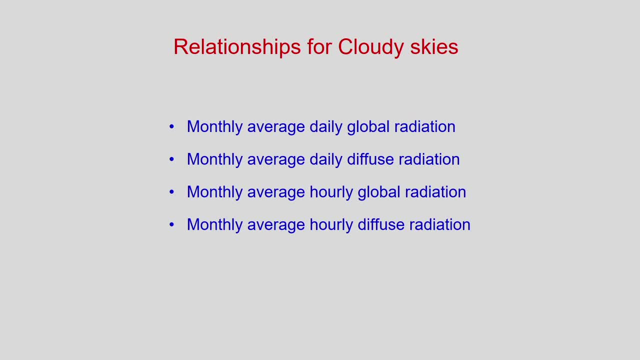 radiation. In the second case, monthly average of daily diffuse radiation. And third case may be monthly average of hourly global radiation. and fourth case may be monthly average of hourly diffused radiation. So we will study all the four cases. So let us first consider the first case, monthly. 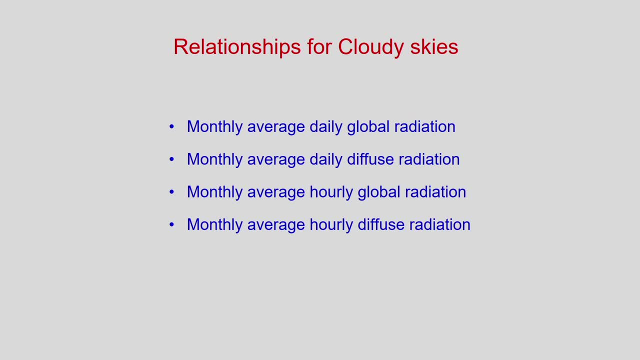 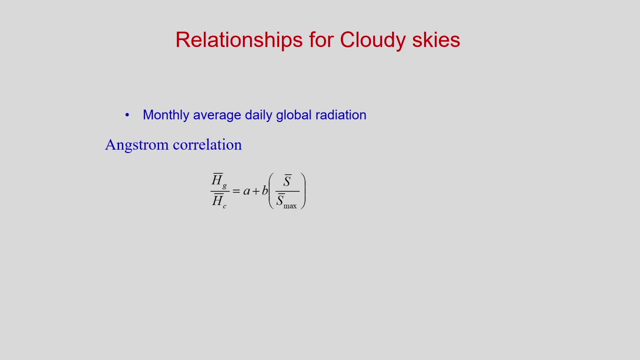 average of daily global radiation estimation. So there are many correlations developed for estimation of monthly average of average of daily global radiations. Among the different correlations, this correlation is developed by Angstrom, which is found to be very accurate correlation, and this is applied to: 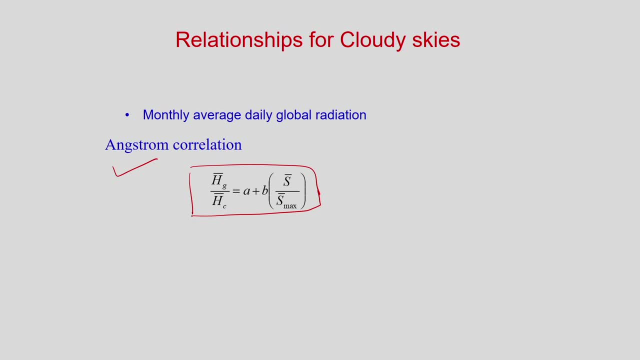 many of the big cities in the globe, as well as different cities of India. And here, what are terminologies used? So Hg, where we need to calculate the monthly average of daily global radiation, and Hc is monthly average of daily global radiations. 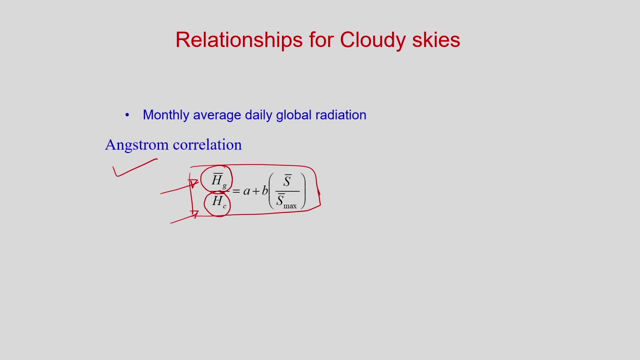 on a clear sky or cloudless day, which is completely sunny days. And these A and B are fitting coefficients and S is the average average of daily global radiations. Hc is the sunshine hour and Smax is the maximum sunshine hour. So this Hc it is very difficult. 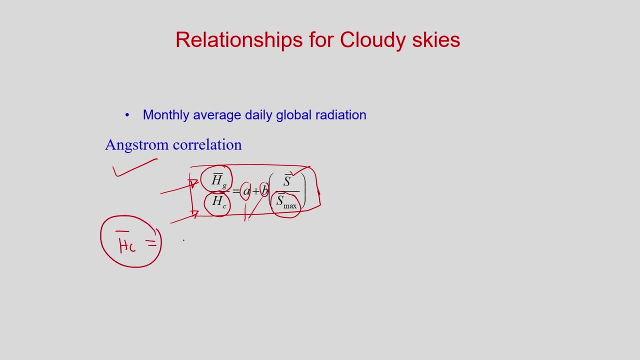 to define what is clear sky. So this is monthly average. so I will write Hc first: monthly average of daily global radiation. and Hc is the average average of daily global radiation on a clear day And these are kilo joule per meter square per day. if I say day, it will be day. 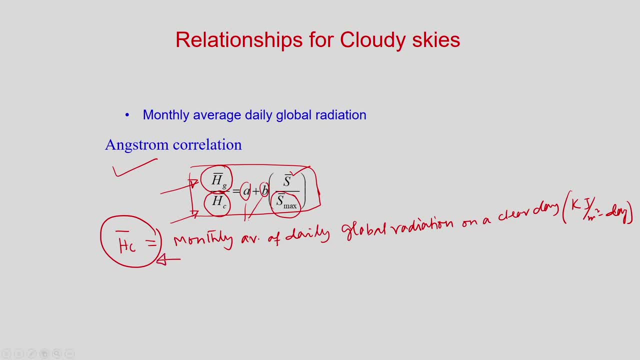 So, as I said, this is very difficult to define What represents clear day. So normally this is replaced by H naught bar. This is nothing but monthly average of daily extraterrestrial region- extraterrestrial region- extraterrestrial region- on the particular day. So this unit is also same. kilo joule per meter square. 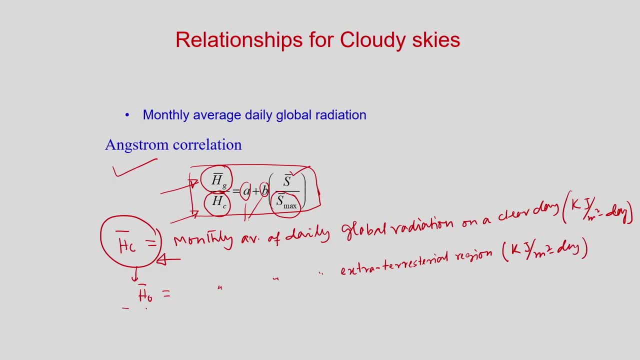 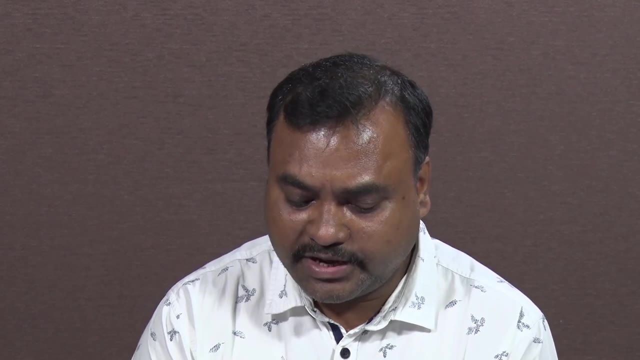 per day. So how to calculate this? This is important, So we will derive the expression for calculation of H naught bar how this H naught bar can be calculated. So this is for extraterrestrial region And, as I said, A and B are fitting coefficient. 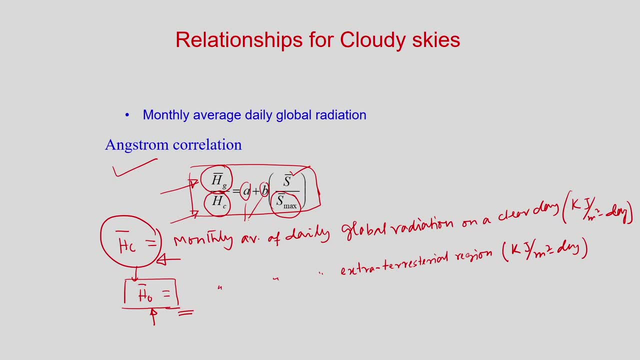 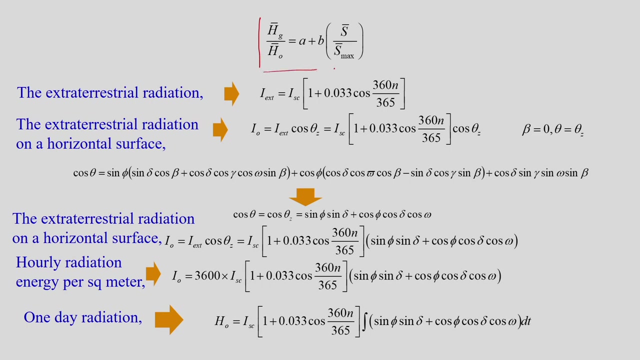 So how this is calculated? By using this radiation, Hg bar data and S bar data. So by using this data, these two coefficients, or regression coefficients, are calculated. So now let us derive the expression for H naught bar. Hg bar to H naught bar is equal to. 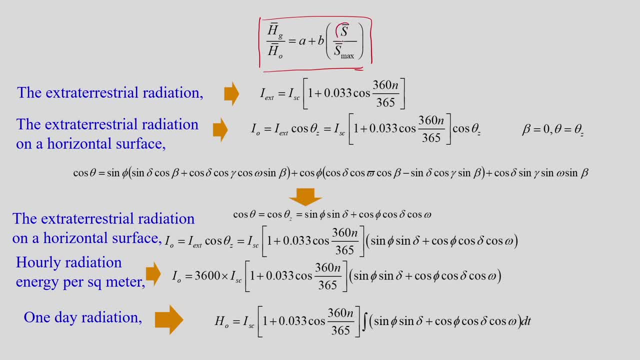 A plus B into S bar, to the S max bar, As you know that these are measured parameters- Hg bar and S bar. So this H naught bar and S max bar need to be calculated. Now let us see the procedure. 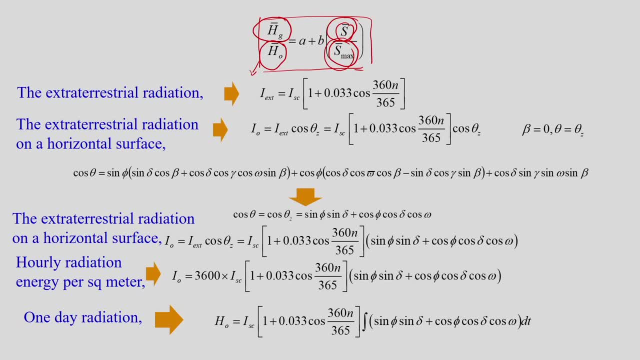 how this H naught bar can be calculated or estimated. This H naught bar is for a representative day, So if, as we, we are aware that H naught is something like radiation in the extraterrestrial region, So as we know, this ext that is, extraterrestrial region, is equal to Isc is. 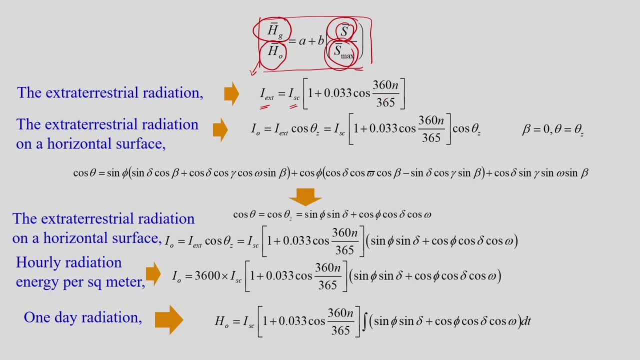 multiplied by 1 plus 0.033, cos of 360n to 365.. So this will be in kilowatt per meter square. So this expression already you are familiar with. Why this 0.033 is present here? all the? 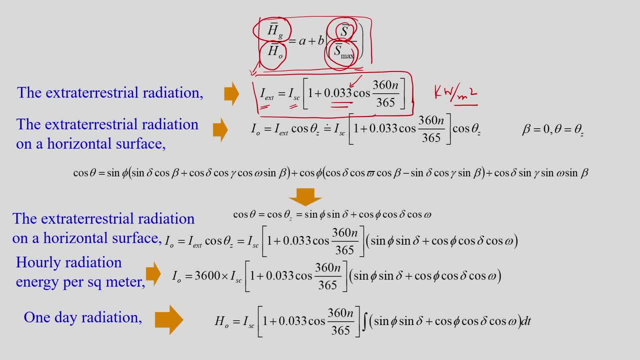 informations are known to you now. So now, if I am interested on a horizontal surface, what is the extraterrestrial radiation? So, for this case, what happens for extraterrestrial region on a horizontal surface? it will be Ext, Ext. 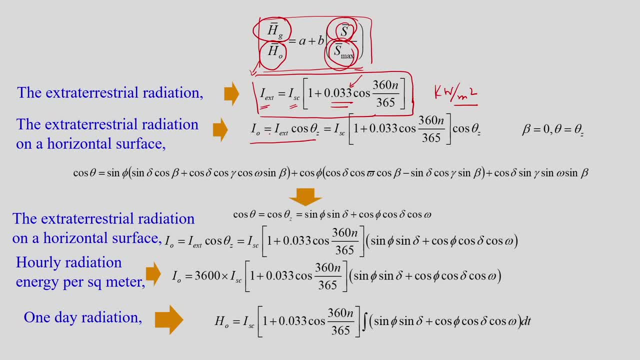 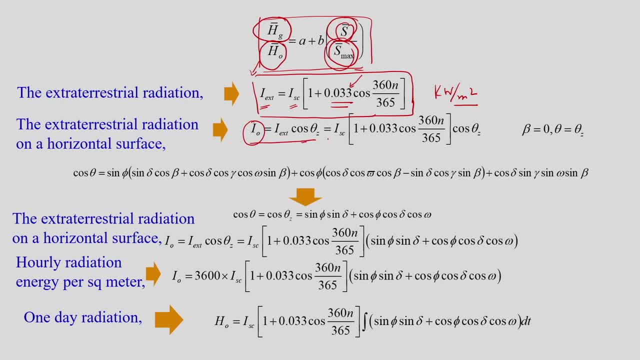 radiation multiplied by cos of theta z. So we can substitute the value of I ext here. So this will be something like this: and finally, this will be multiplied by cos of theta z. So for a horizontal surface, what will happen? beta will be 0.. Beta means slope will be 0,. 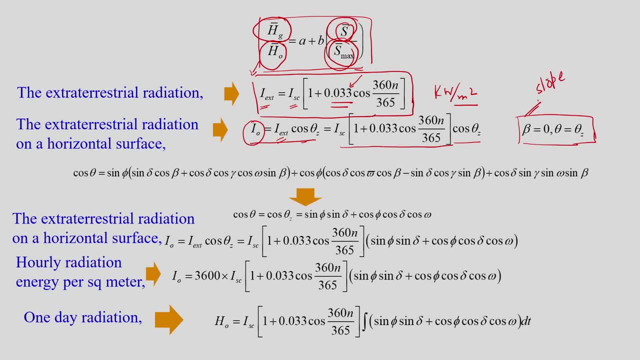 this beta is nothing but slope. So if, for example, this is the surface, so this is represented by beta, so beta will be 0 for a horizontal surface And of course this theta is equal to theta z. what is theta? 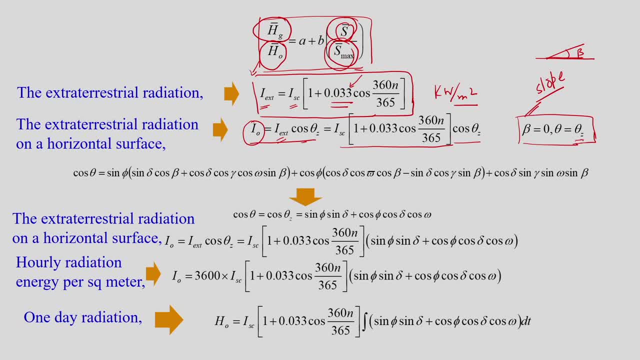 Theta is. angle of incidence is equal to azimuth angle. So because of that we can represent this cos of theta z. So if we substitute beta is equal to 0 and theta is equal to theta z, then our expression will be something like this: 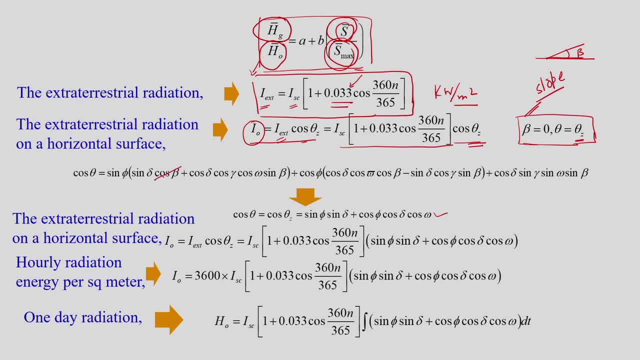 So here, if we substitute beta, value is equal to 0, so cos beta is 1.. If it is 0, so sin beta, this part will be 0. And then again this part will be 1, then sin will be 0 and 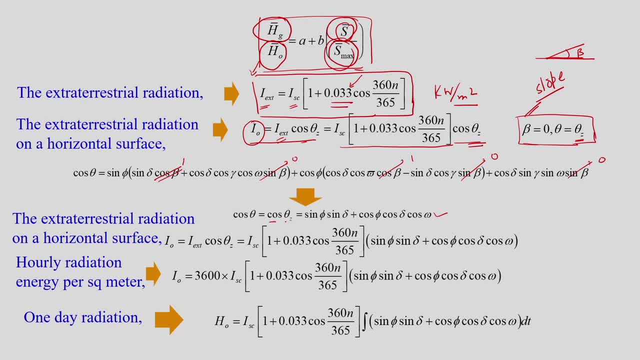 again, this will be 0.. So, finally, what we will have this: cos theta z is equal to sin of phi, sin of delta, plus cos of phi, cos of delta and cos of omega. Okay, which is nothing but our angle. So these expressions we will get when we substitute: 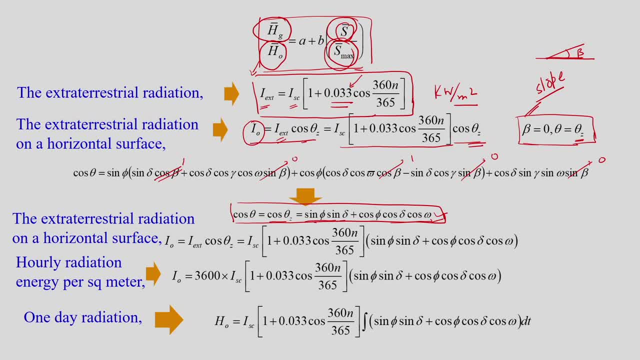 slope or beta is 0 and theta becomes theta z. So this is the expression. Now, if I am interested to know the extraterrestrial radiation on a horizontal surface, then we can substitute this value, cos, theta z, what we have found here in the equation. 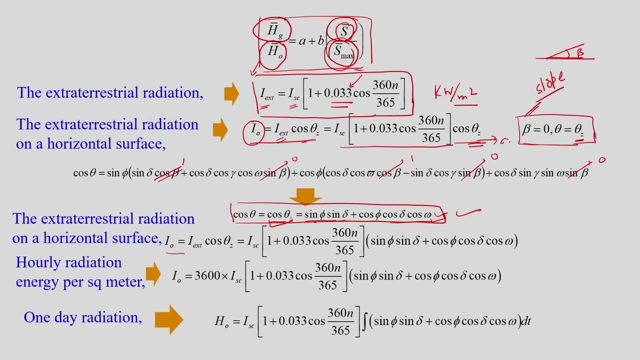 maybe we can write this equation as a. So if we substitute the cos theta value in the equation a, then our equation will be something like this. So this equation we will get. So this maybe we can write as b. And now if we are interested in hourly values: 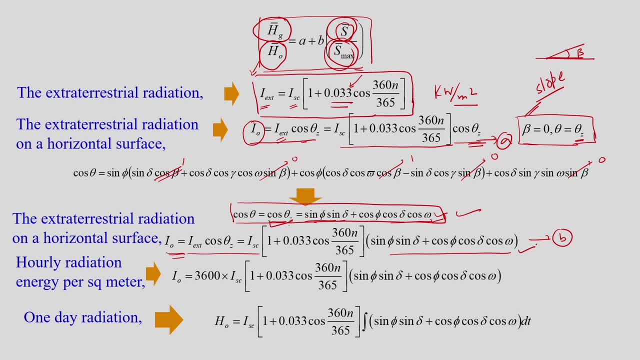 these values are instantaneous. So if we are interested to know hourly values, then what we will do: We will multiply this expression with 3600.. So this will become like kilojoule per meter square. this is hour, And again for a day. if we are interested, then what we will do: We will integrate this time from. 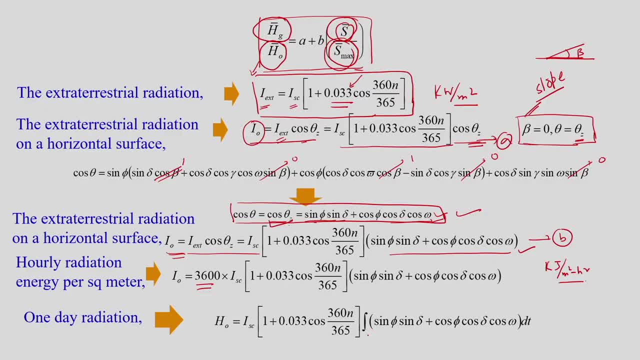 morning to the evening. So this is what we need to do: the calculation. So, for a day, what we will do- H naught- we will represent this by H naught and we will integrate this equation with C And then what we will get is the radiation received on a particular day. 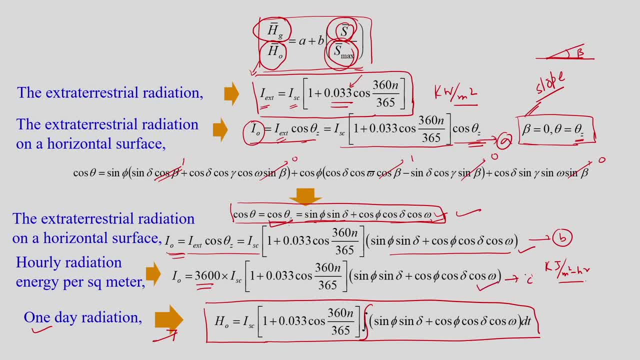 So here this expression is for hourly, So we can represent this equation as C And this equation is for daily, So we can represent this equation as D. So for daily radiations we will follow this expression and for hourly variations we will follow this expression. So why this kilo here? So 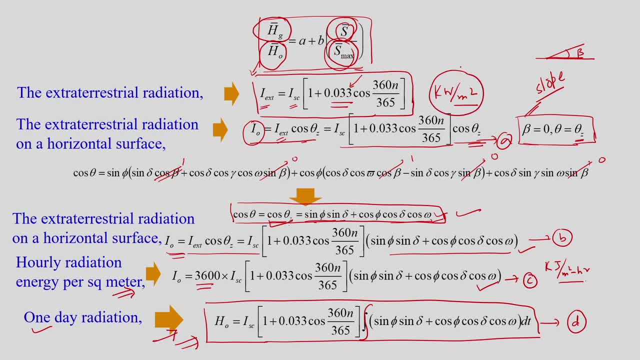 why we are writing kilowatt per meter square? Because this ISC value. ISC value, as you already aware, 1367 watt per meter square. if we write kilowatt per meter square, it will be 0.367 kilowatt per meter square. That is why it is represented in kilowatt per meter square. and then when we 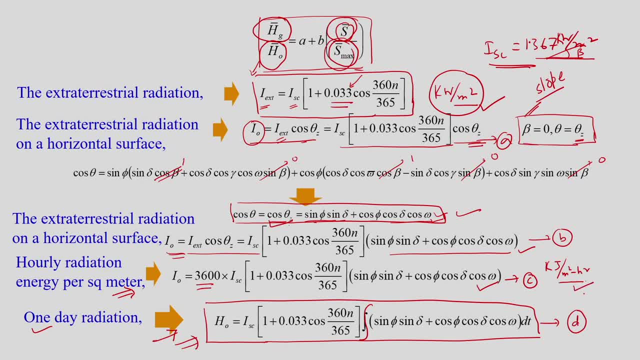 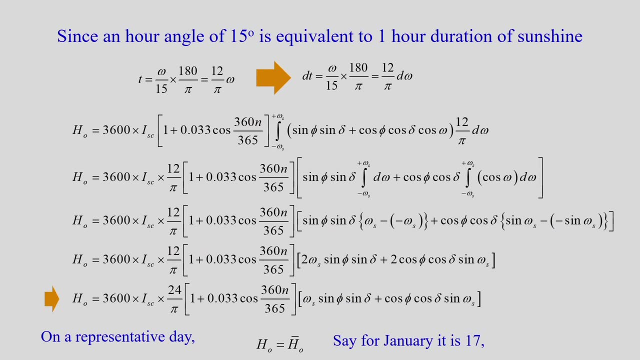 multiply 3600, it becomes kilojoule per meter square per hour, And for daily basis it will be kilojoule per meter square per day. So this is how units are used for expressions. Now let us do it for when we integrate. so we need to integrate over this omega, and then we 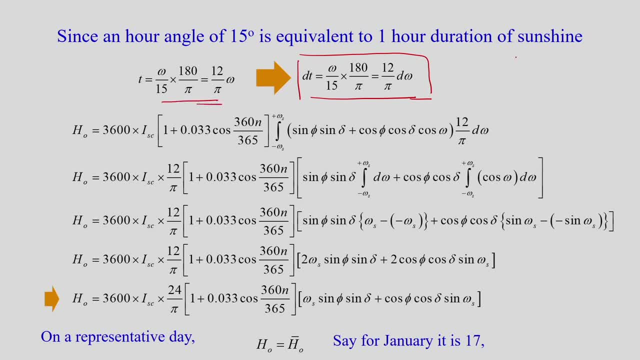 have to convert this, as you know, if we have to convert degree to radian, So one one degree is equal to pi by 180 radian, 180 radian and maybe one radian is equal to 180 by pi. So this is in degree. So we know this before and we can apply this concept. 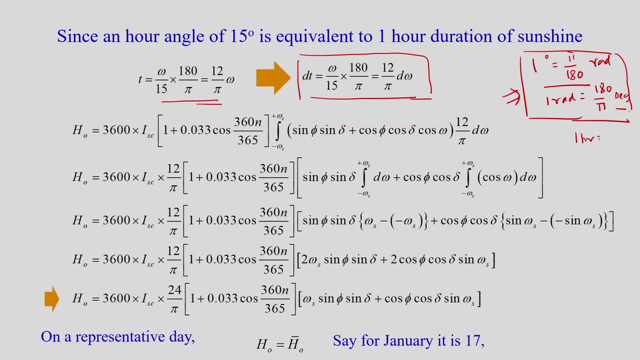 and also we know one hour is 15 degree. That means that an hour angle of 15 degree is equivalent to one hour duration of sunshine hour. So this knowledge we need to apply here for integration. so what we did, this T is in hour. 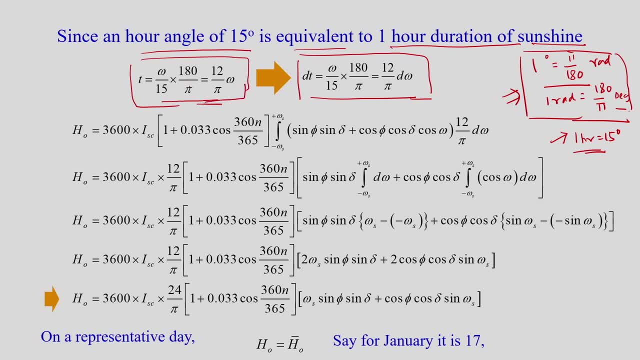 and omega is in degree, and then you have to convert to radian and then already we know this: 15 degree is one hour. So what we will get here, this part is in hour. So dT will be omega by 15 into 180 by pi, and then, if we simplify it, it will be 12 by pi of radian, and then wait till. 18 minutes and we have divided by pi, times 12 by pi, So that is the number of units that we have. this is a quarter hour. hear about it in 12 minutes. So in the next part we are going to have dT, which means 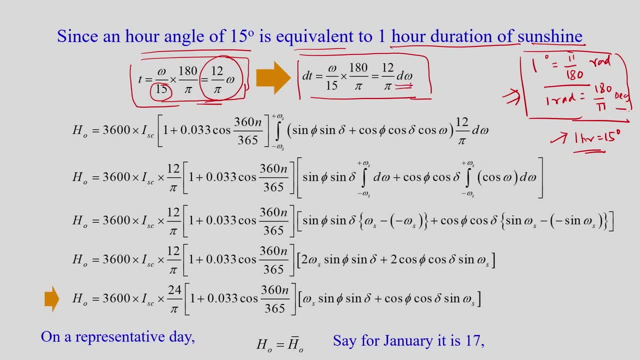 And then, if we simplify it, it will be 12 by pi of d omega. So now sense of integration. so it will be minus omega to plus omega. So if we use the earlier equations and we do the integration, then what we will get? We will get something like this. So this part. 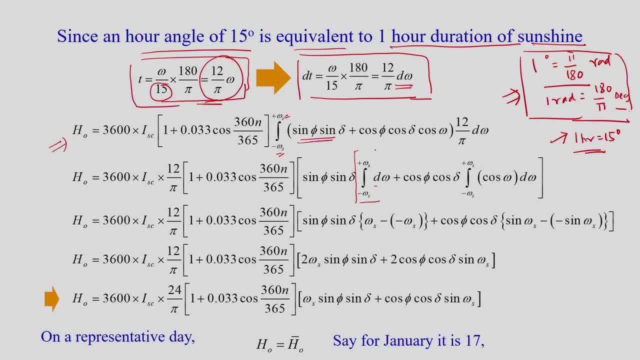 is constant. So we have to integrate over omega. This is our angle, and then this part will be something like that and this is constant. So if we do the integration, then finally what we will get This will be 2 omega multiplied by sin phi, then sin of delta plus 2 of cos. 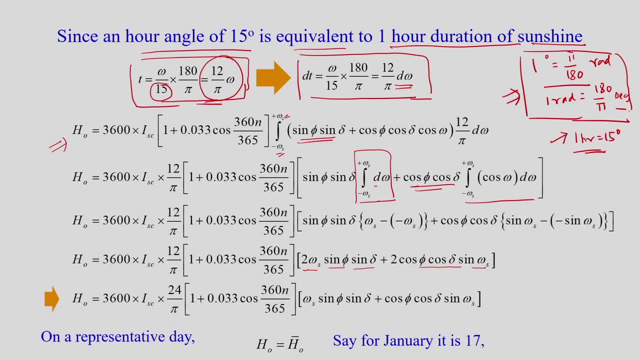 of phi, cos of delta, then sin of omega s. So we can take out this 2 from the bracket and then we can multiply. it will become 24 by pi. So this is the expression for calculation of H naught. So this expression we need to use for calculation. 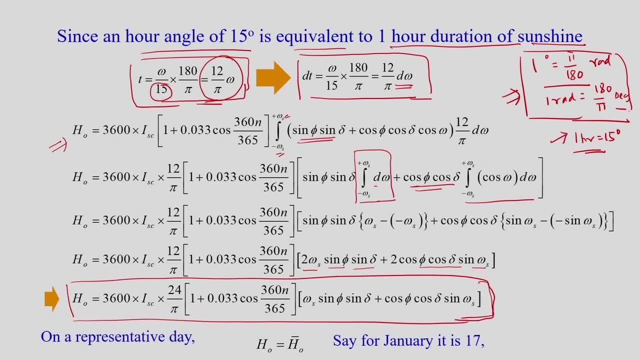 of radiation, radiation received on a particular day in the extraterrestrial region if the surface is horizontal. So, as we know the recommendations provided by Klins, that on a representative day, that maybe if we consider January, then 17th of the January is known as the representative day. 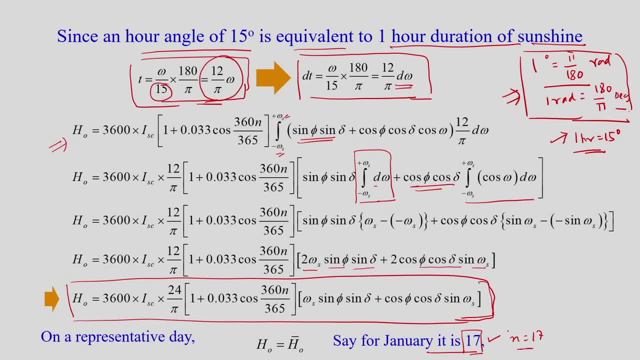 and on that day so n will be 17.. So if we substitute the value of n here in this expression, then what we will get We will get the monthly average of the daily terrestrial radiation. So under that condition, what we can do, We can replace this H naught by H naught bar. So 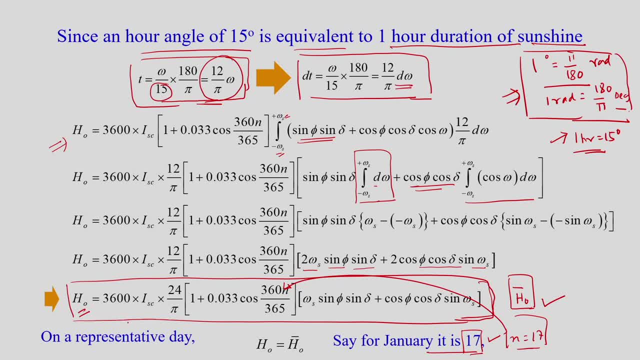 that is how we can get the H naught bar. Otherwise, we need to do the calculation from day 1 to the day 31 for the month of January. So, since people have done a lot of research on this and finally they have recommended a day which represents the particular month, so we can take. 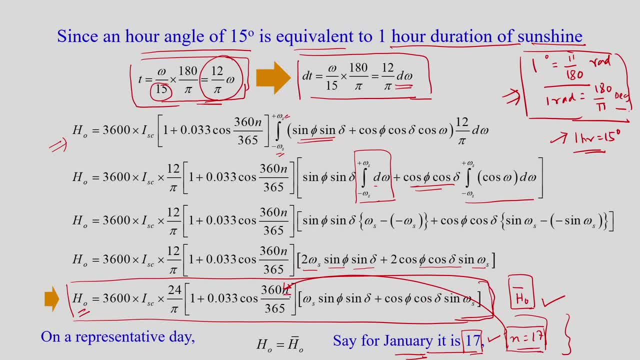 straight away that number And we can substitute the value here in the n, and under that condition this H naught will be converted to H naught bar and this will represent that monthly average of the daily extraterrestrial radiation. So once we know, then we can do the calculations for Hg bar. we can calculate which. 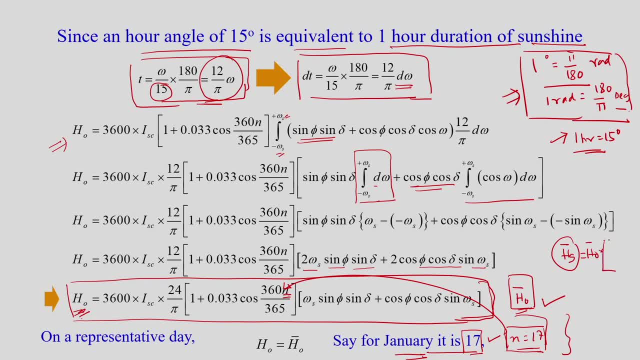 is nothing but H naught bar multiplied by. if we use that angstrom correlation, a plus b s, by s max. So we can use this correlation and we can get the value of Hg bar. So this is the procedure. 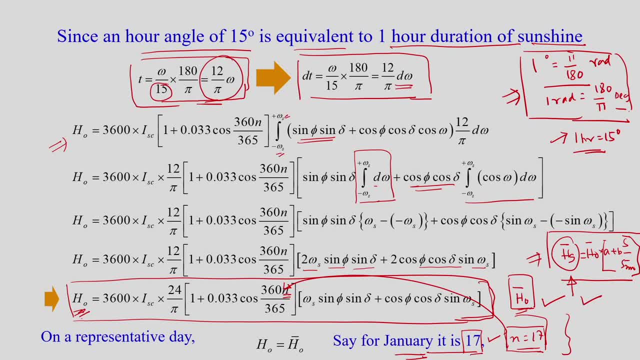 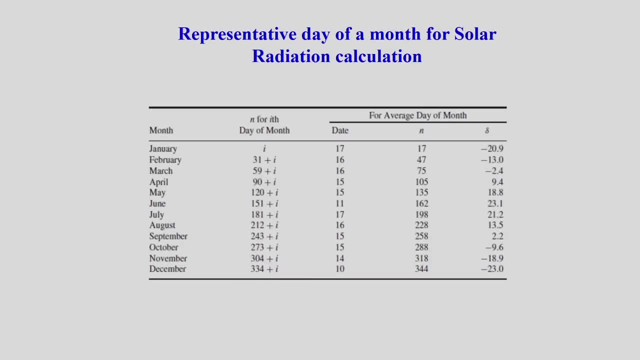 by which we can calculate monthly average of daily global radiations on a horizontal surface. So these are the recommendations made by different researchers. So if we consider January, then 17th of the day we can consider, On that day we can say H naught is equal to H naught bar. So that way we can. 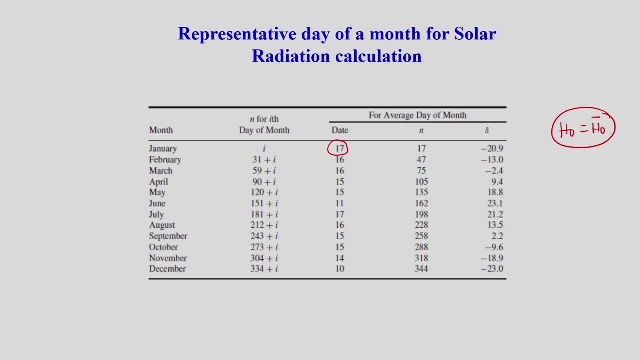 consider for all the other months. So, for example, February, it will be 16th. 16th of February will give the radiation spectrum of on the particular month. So that way we can, we can do it. So this figure has already been discussed in the last class. So on particular day. 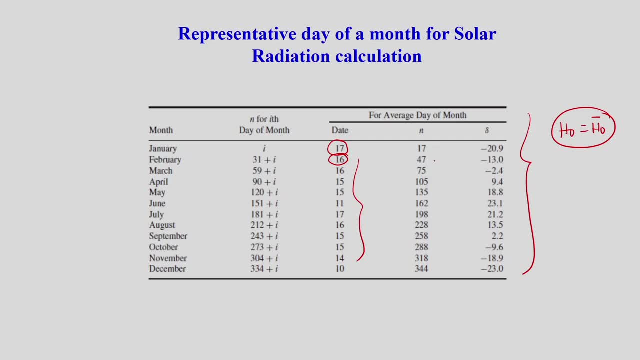 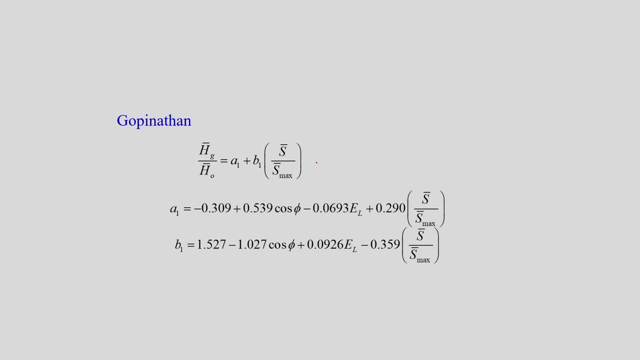 we can say how this declination varies and what is the value of n. So that way we can do the calculations and we can estimate the radiation properties. Now let us see the other correlations developed by other researchers. This is one of the correlations developed by Gopinathan. 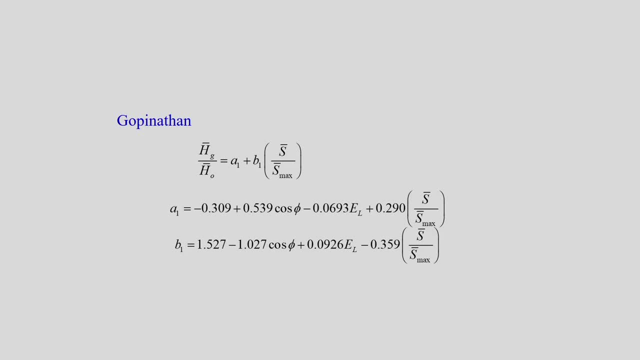 So what he has done, he has taken about 40 cities and he has collected many informations. apart from radiation and meteorological data, He has incorporated one more parameter called elevation. So what he has done, he has used phi, then elevations, El and then solar. So this: 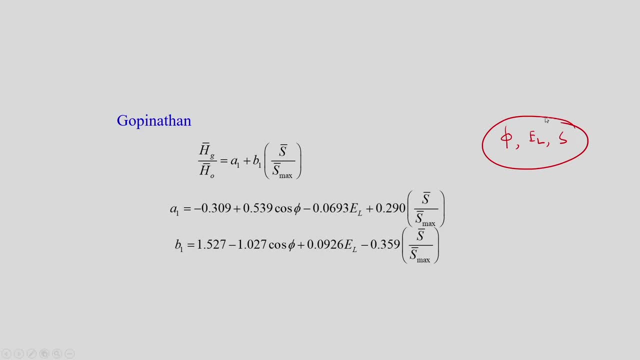 day length or say sunshine hour. So these values he has considered and he has used these values for calculation of a1 and b1. So by considering this we can finally calculate what is the monthly average of daily global radiation on a particular place. So procedure for calculation of H naught bar is same. 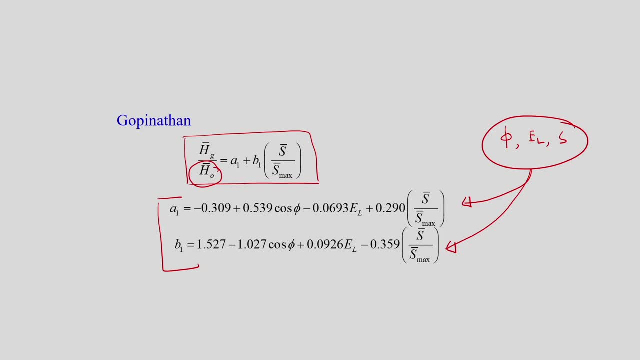 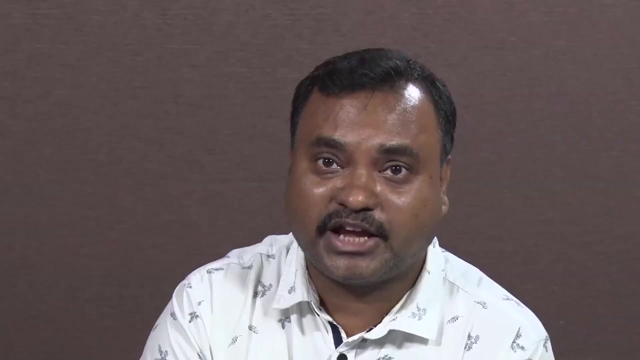 as what we have discussed before, and we can see how this Hg bar varying with time. If we know or we can say we can compare the values given by Gopinathan and the results given by the angstrom correlation So that can be compared. 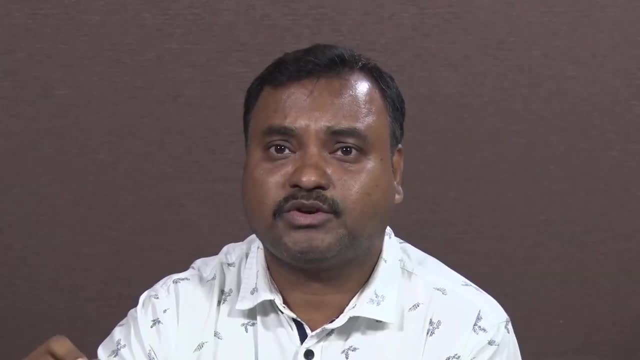 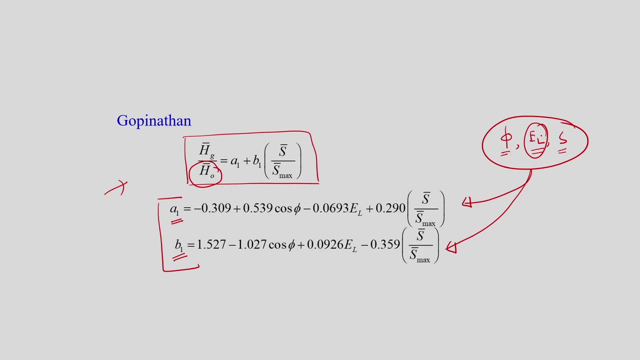 So, apart from sunshine and precipitation, what was considered in angstrom correlations, here one more parameter, that is El, was introduced and finally, this regression coefficients were calculated. These were functions of phi, El and S. Anyway, this S max can be calculated. 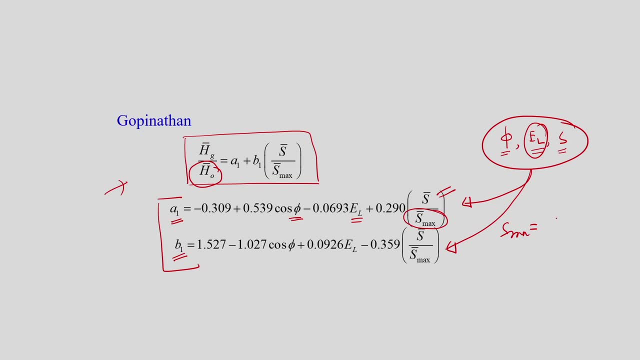 Based on, as we have understand this, S max is cos inverse of 2 by 15, cos inverse of minus 10 of phi, and then you have 10 of delta. So by using this expression we can calculate what is S max. So, in summary, what we can say, there are many correlations. 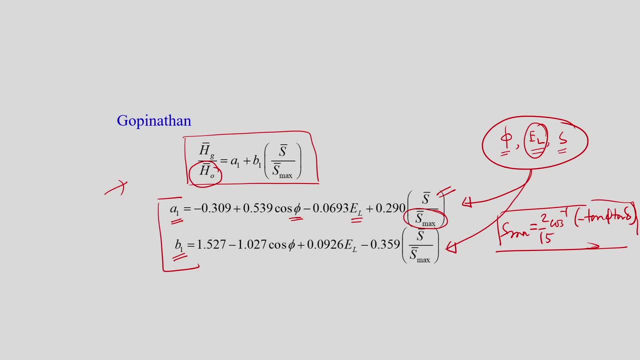 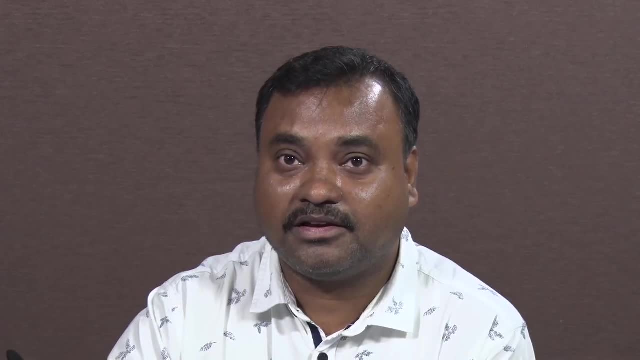 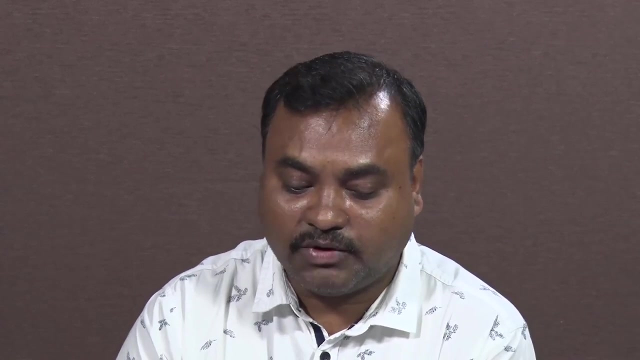 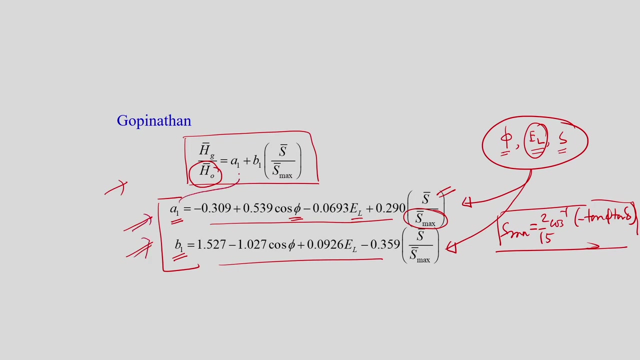 Gopinathan has developed one more correlations by introducing other variables and considering more datas and he has found this: a1, b1 are related with these expressions And once we calculate a1 and b1 on substitution of those results here in this expression, and since we know 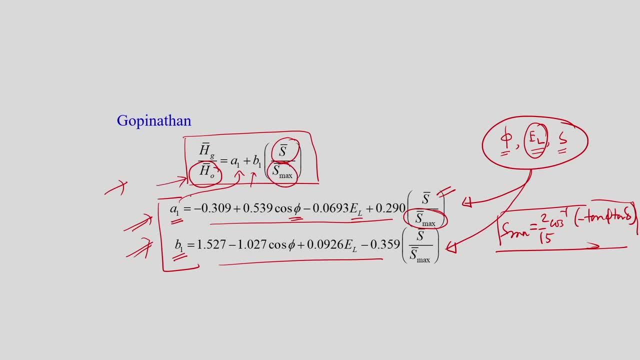 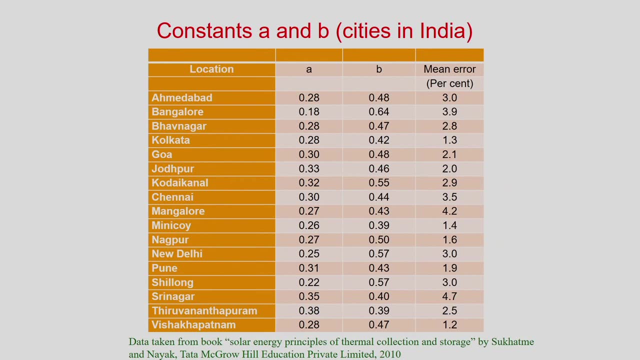 this and we have calculated this and this can be calculated, what we have defined just now. then, finally, we can calculate what is Hg bar. So, without further delay, we can solve one problem to understand our understanding on how to estimate monthly average of daily global radiation. So this chart is required and this chart was taken. 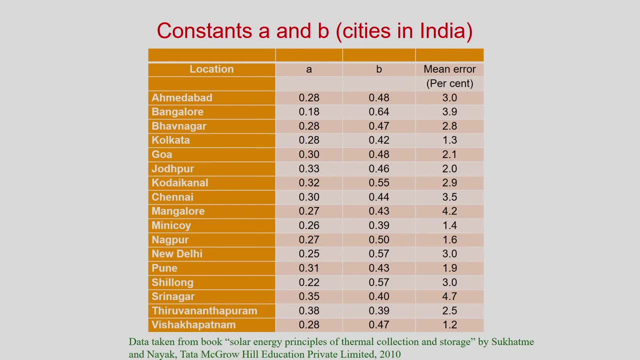 from solar energy principle of thermal collection and storage by Sukhatme and Nayak, and these values were reported. So for different locations we will have different values of a and b, So which locations we are targeting to calculate the radiation or to estimate the monthly average? 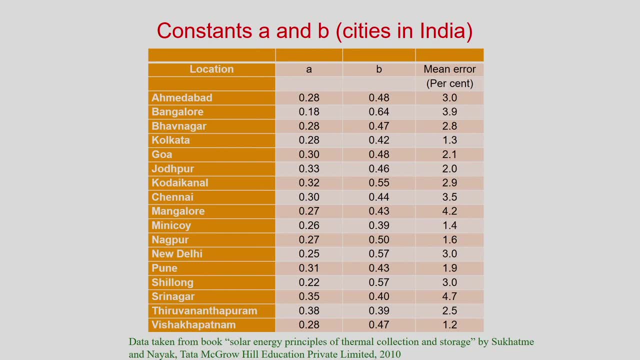 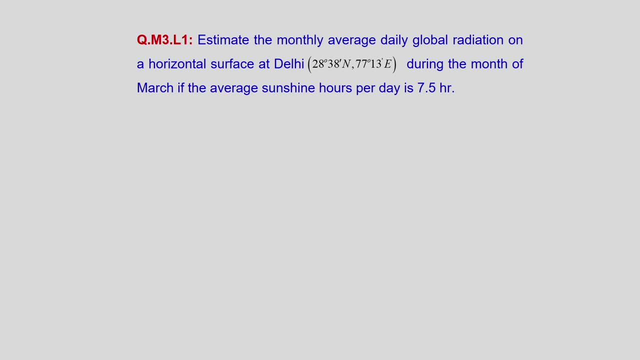 of daily global radiation. So that way we can take the data and we can do the calculation. So let us take this example: like we need to estimate the monthly average of daily global radiation on a horizontal surface, say at Delhi, So its latitude and longitude are given, and month. 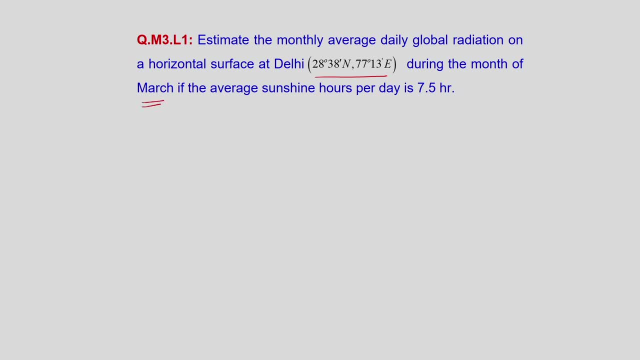 for which we need to calculate is March, If the average sunshine hour is given as 7.5.. So here what we can say. so solution goes something like this: So we will have phi, latitude we need to calculate because 28 degree and then we have 38 divided by 60. So this will give you phi and each value will be 28,. 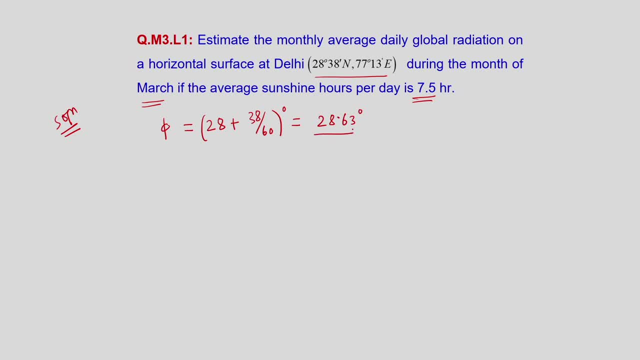 point 63 degree, as per my calculation, and as it says we need to estimate the radiation or global radiation for the month of March. So it is not said the date. So we must know which date we need to calculate. we need to follow this chart If we need to calculate. 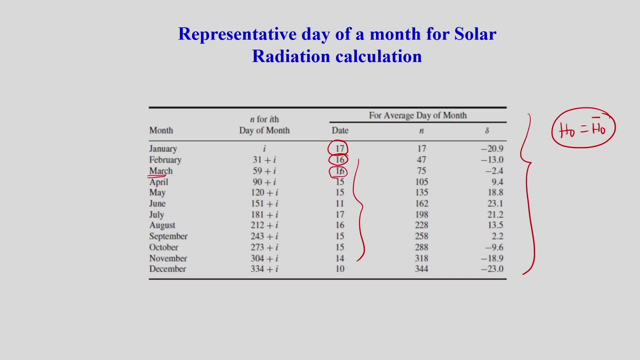 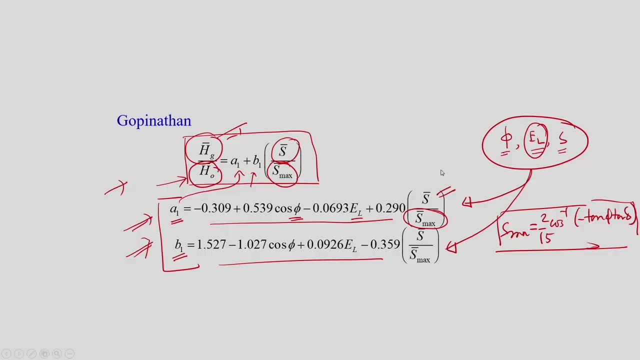 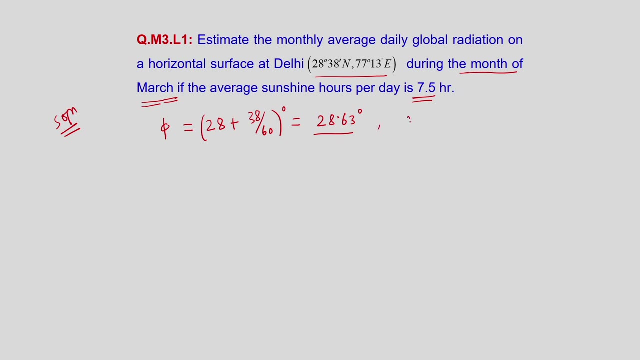 for the month of March, then that will be on 16th of March and the annual will be 75. So what we will do here now, so March 16,, so March 16, and then finally n will be 75. Or 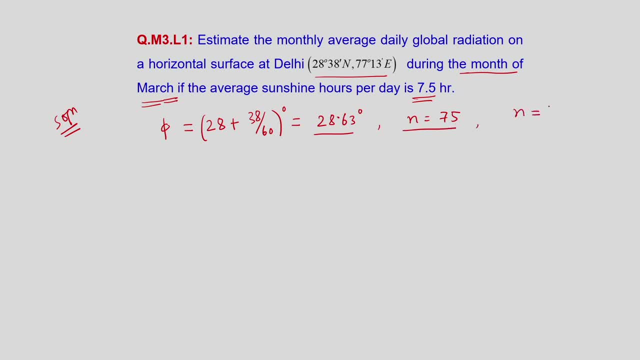 otherwise we can calculate what will be n. So starting from January, January is 31,, then we have 28,, then we have March 16. So if we add it, then it will be 75. So once we know n, then what we can calculate, We can calculate what is delta, because 23.45. 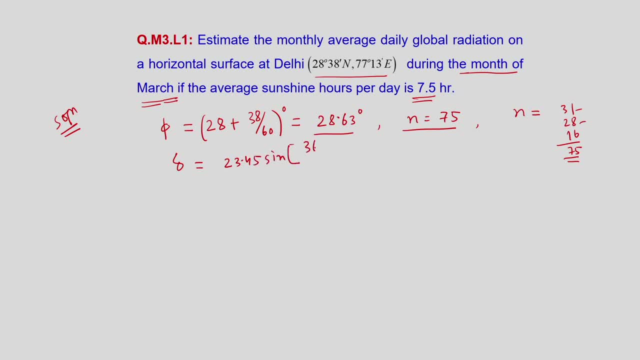 sine of, we have 360 by 365, then 284 plus 75. So if we substitute this value, then what we will get, delta value will be minus 2.42 degree. So now we know phi and delta and S is given. so S, what is the value of S? S is given as 7.5 hour, 7.5 hours. 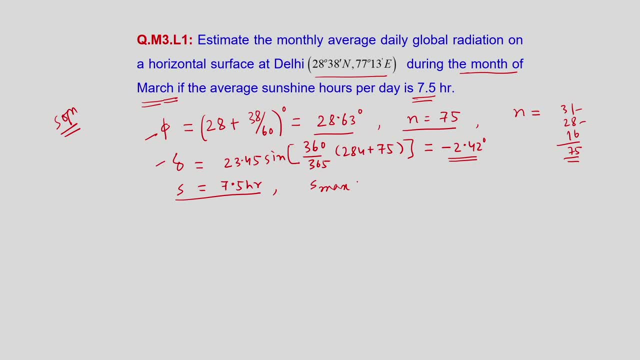 So we can calculate S max. How to calculate X max? We know 2 by 15 of what is known as cos, inverse of minus 10 of phi. then we have 10 of delta. So this phi and delta is known. 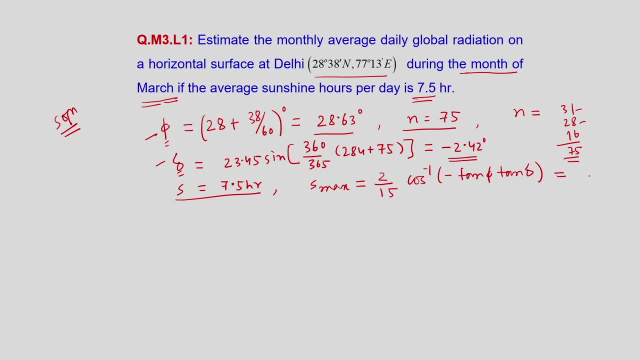 one of solutions. what we will get, S max or del n, will be 11.82 hours, and this is nothing but del n. Also, this is nothing but omega S. So what is omega S? So omega S value will be cos inverse of. 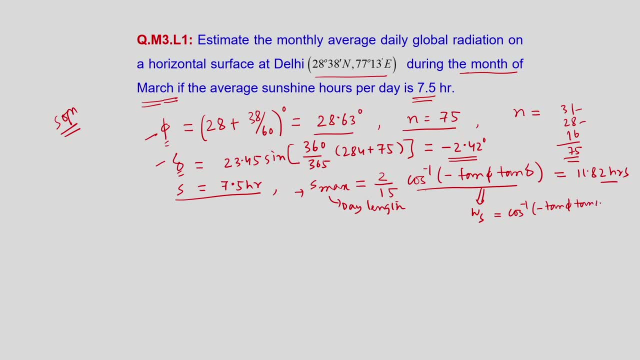 minus 10 of phi, then we have 10 of delta. So once we substitute the value of phi and delta, then what you will get is omega S and, as per my calculation, it is about 88.678 degree. And if we have to convert to radian, then we can convert it to radian: it will be 1.546 radian. 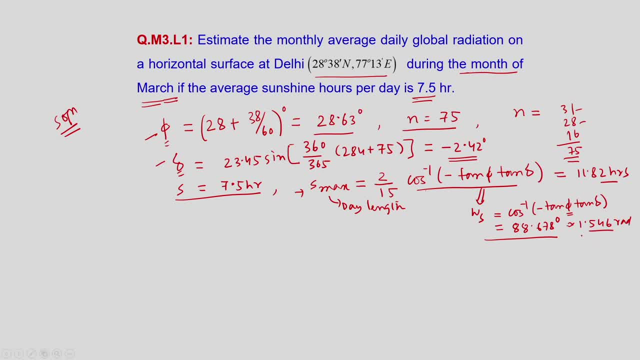 So you know how to convert degree to radian. So if we have omega into pi by 180, then it will become radian, So that way you can calculate it. So once we do omega S, then then next calculation will be over H0 bar. So how to calculate this H0 bar Already? 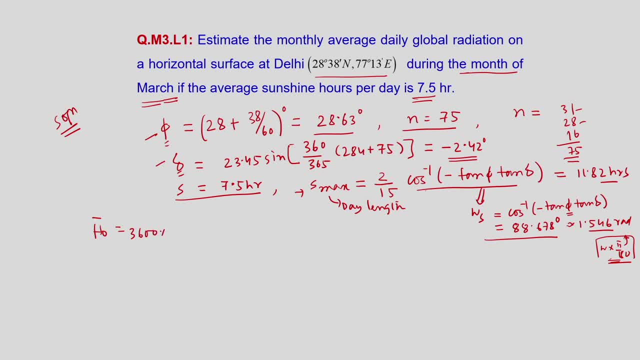 we have derived the expression So 3600 into we have 24 by pi, and then we will have ISC, and this is 1 plus 0.033 cos of 360 divided by 365 into n. This, multiplied by, will have omega S sin of phi. then we have sin of delta plus cos of phi. cos of delta. 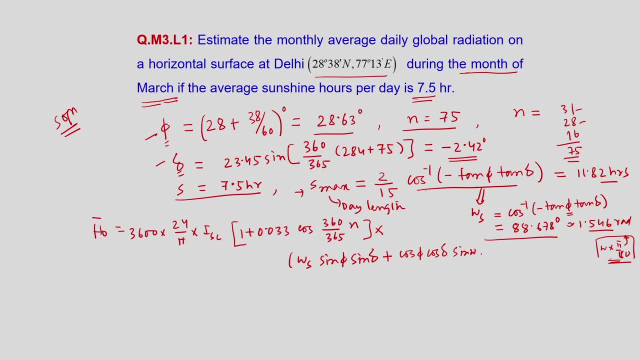 delta, then we have sin of omega or omega s. Now, if we substitute the value of n, n is equal to 75 days and all the values of angles are known to us now. So we can substitute here and here we need to substitute 1.367.. So this will be in kilo joule per meter square. 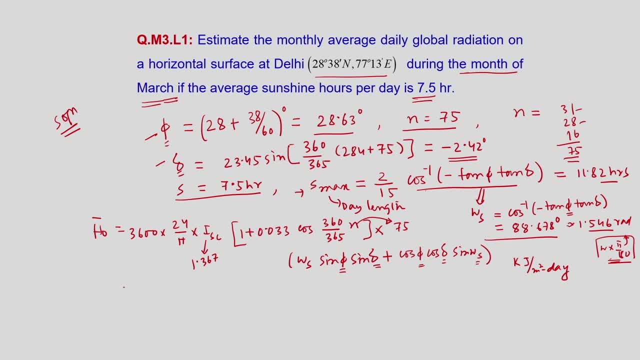 per day. So if we substitute these values, then what we will get is, as per my calculations, I got it 31784.37 kilo joule per meter square per day. So this is H naught bar. this is the monthly average of daily extraterrestrial radiation on a horizontal. 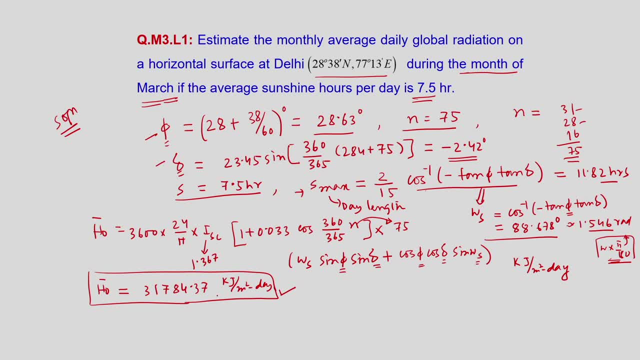 sphere. So this is H naught bar on a horizontal sphere and this is H naught bar on a horizontal surface. So since we know this value now, we can use this angstrom correlation: Hg bar to H naught bar is equal to a plus b s by s max, So we can put a bar on s and s max. 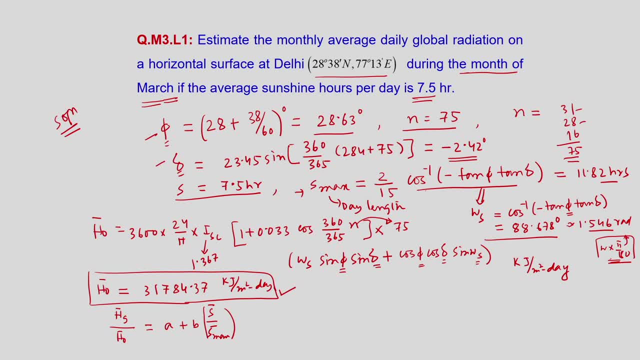 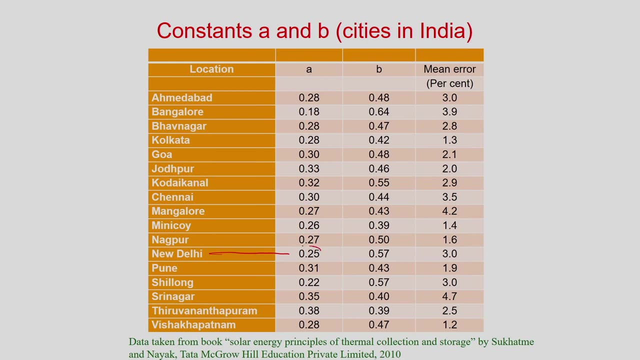 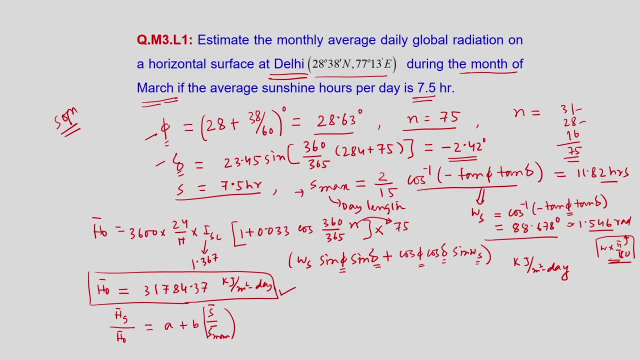 So this a and b values. so this we can use the earlier chart that we have discussed. So what will be the values of a and b for daily? Lets us see this So we find out the daily. So here is the daily, and A value is 0.25 and b value is 0.57, okay, So if we substitute 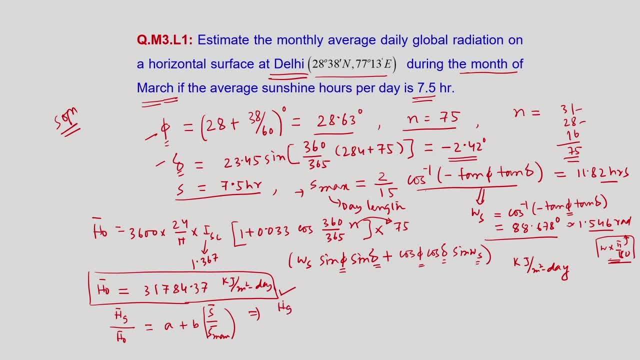 these values. so is g bar. we need to calculate This is just one. Get this value. So this a and b values. so x r bar is equal to a to 2 and y was equal to 0.リ env and b value was the 0,506,. okay, So you can multiply this. gger and recommend this value 1200.. Will I QUESTION E назад to find out those values? And this is played through this problem. if you have 16 prime 반, the infinity given, Alright. So if we substitute these values, so hg bar, we need to calculate. the value is going to be as: 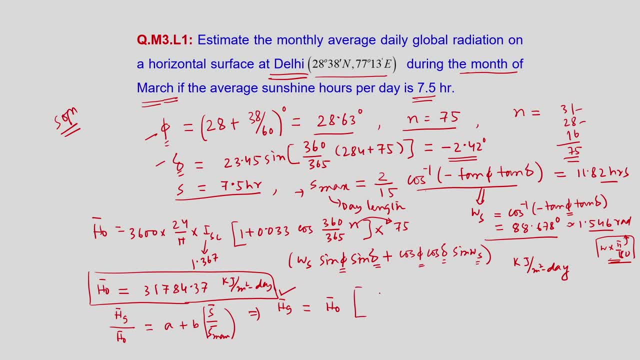 equal to H naught bar, then A is 0.25 plus we have B is 0.57, then we have S. S is how much? 7.5 hours? then S max is already. we have calculated what is S max is 11.82 hours. So 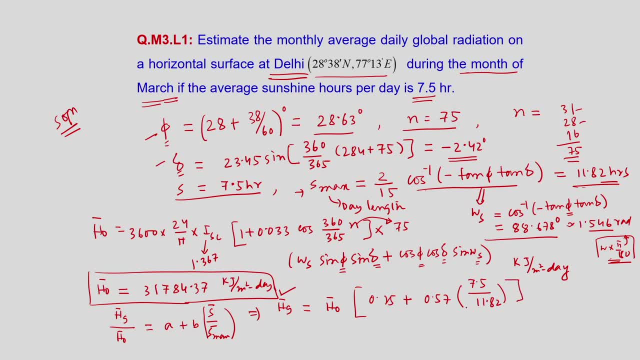 this hour, hour cancel. so this becomes kilo joule per meter square. then this: So if we substitute the value of H, naught, which is equal to 131378.37, 784.37.. So if we substitute here and we do the calculation, it will be: 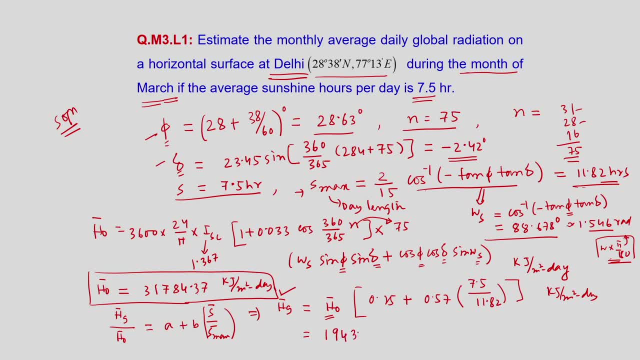 19438.37.. This will be kilo joule per meter square per day. So this is the monthly average of daily global radiation received on a horizontal surface on the earth. So this is the procedure: how we can calculate the monthly average of daily global radiation on a particular place on the. 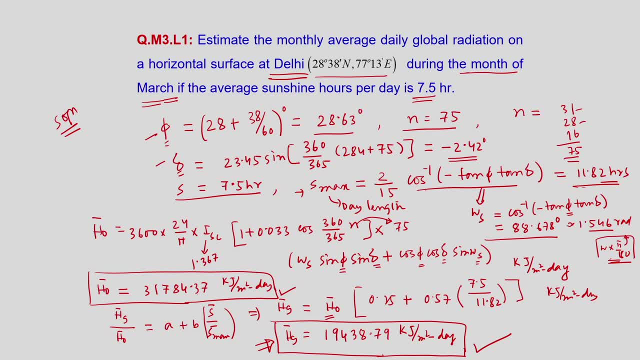 earth. So what we did in the problem: first we try to see what is the latitude and then we have converted this to degree and n we have calculated, because for the month of March we know what is the value of n, and then we can calculate delta, and S is given.